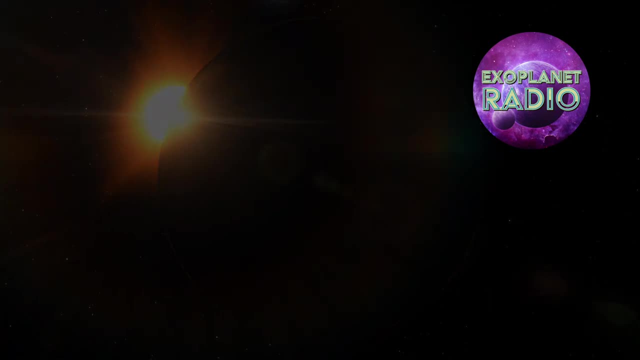 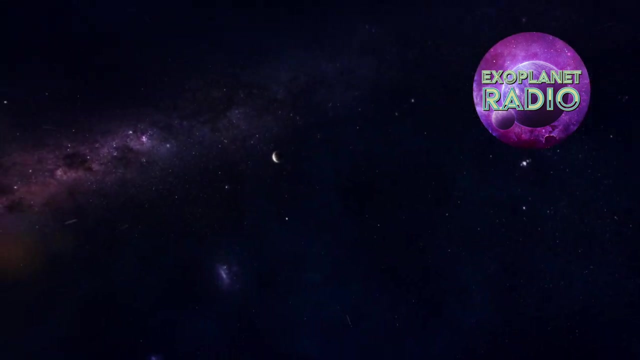 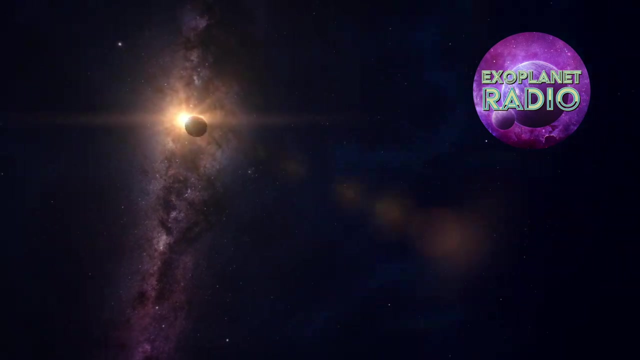 This is unimaginatively called the direct imaging method and has revealed some amazing results. So here's the scenario: We see all planets, including those in our solar system, in reflected light from the star. Starlight shines on a planet and is reflected to our telescopes. 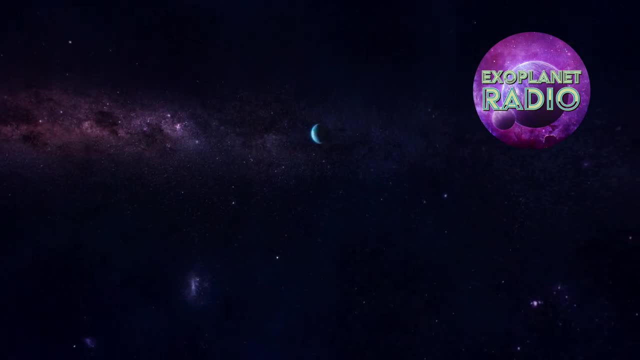 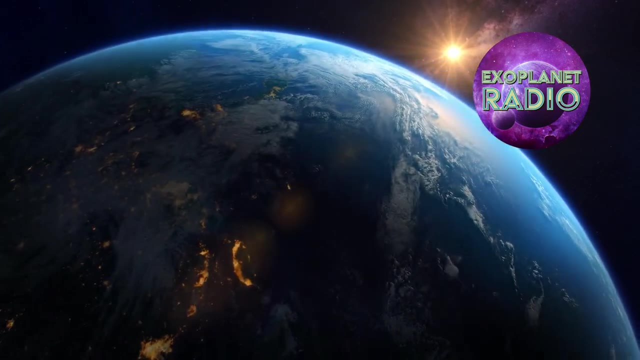 Now imagine trying to see a tiny speck of dust right next to a very bright light bulb. This is the challenge of direct imaging: planets light-years away. The star's light is so dazzling that it blinds us from seeing the planet's faint glow. 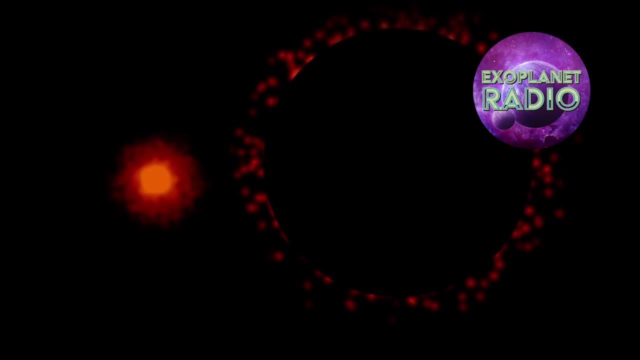 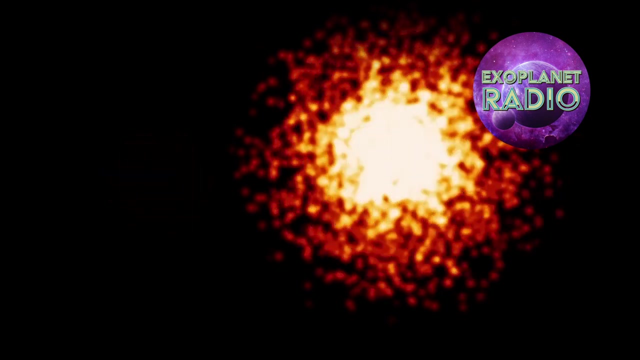 To fix that, astronomers use a special device called a coronagraph, which blocks out the star's light and lets us see the planet's reflected light. Using this method, astronomers have captured some stunning images of exoplanets such as 2M1207b, the first exoplanet to be directly imaged. 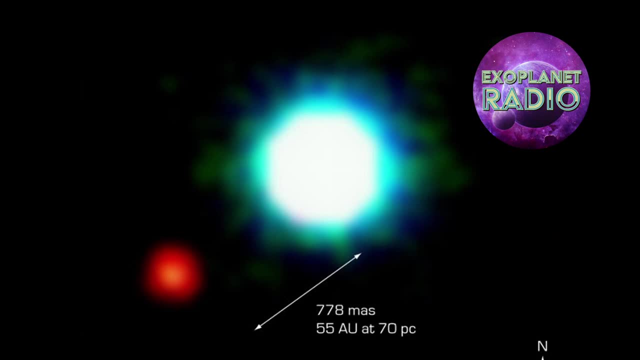 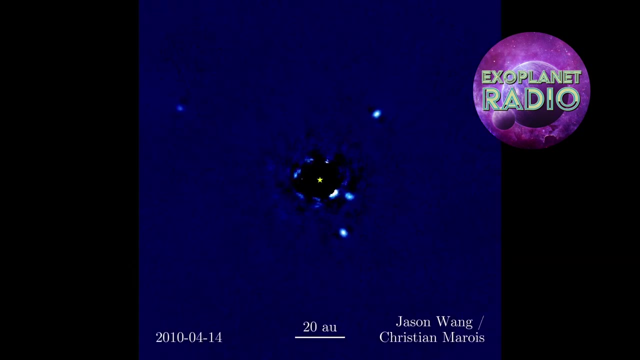 and also the first one to orbit a brown dwarf star, a failed star that's too small to shine. We have also seen four planets orbit around the young star HR 8799, in a mesmerizing choreography. Direct imaging is not only beautiful, but also powerful. 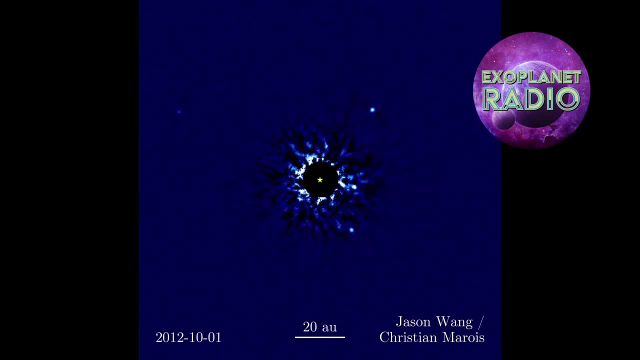 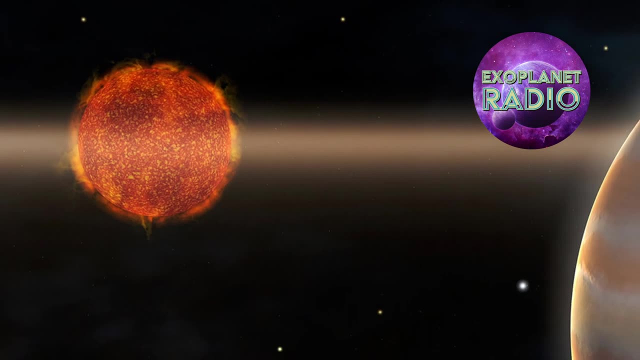 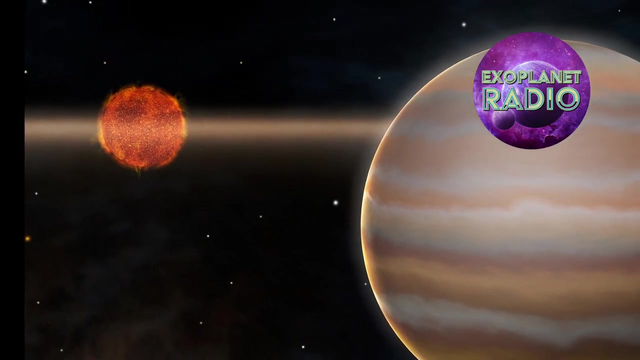 It can tell us more about exoplanets than any other method. It has the potential to show us their colors, shapes, sizes and even their weather patterns. It can reveal their oceans, continents and maybe even signs of life. It can open our eyes to new worlds and new possibilities. 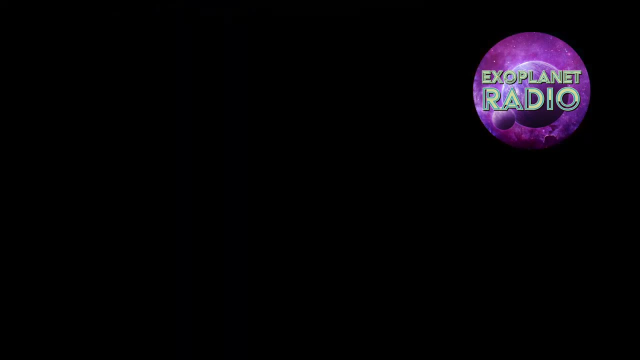 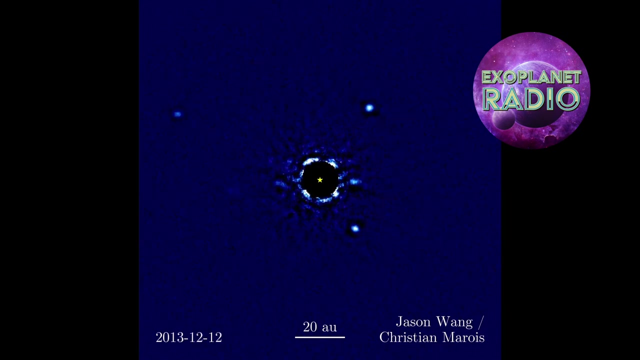 Direct imaging is the ability of our intelligent eyes to see knowingly. Direct imaging is still a young and evolving technique, but it has already shown us some of the most incredible sights in the universe. As our technology improves, we will be able to see more and more exoplanets with direct imaging. 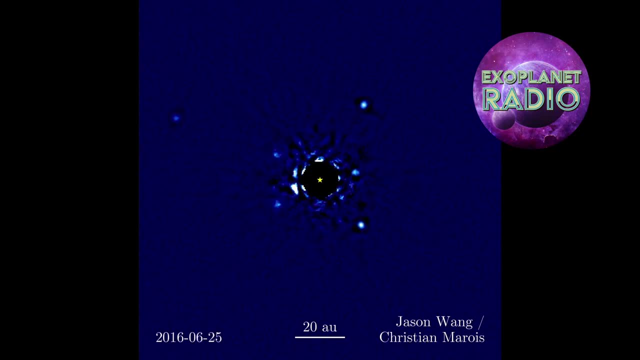 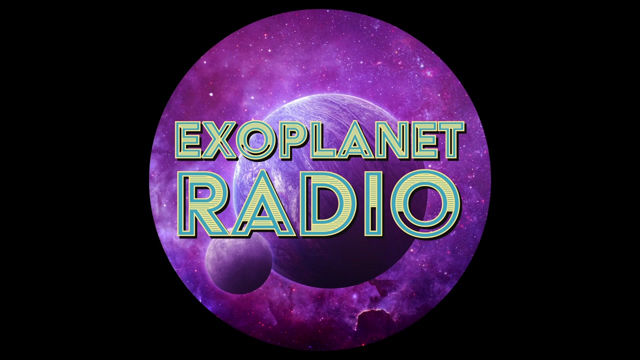 and learn more about them, We will be able to witness the diversity and beauty of these distant worlds, and maybe even find one that is like our own. Exoplanet Radio is produced by Deep Astronomy. The music was composed by Geodesium and available at LochNessProductionscom. 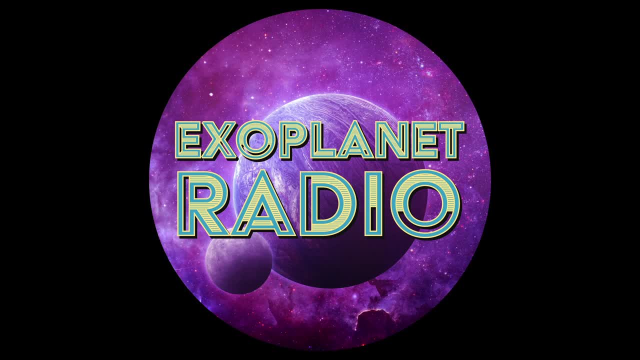 Get all episodes from ExoplanetRadiocom or anywhere you get podcasts.